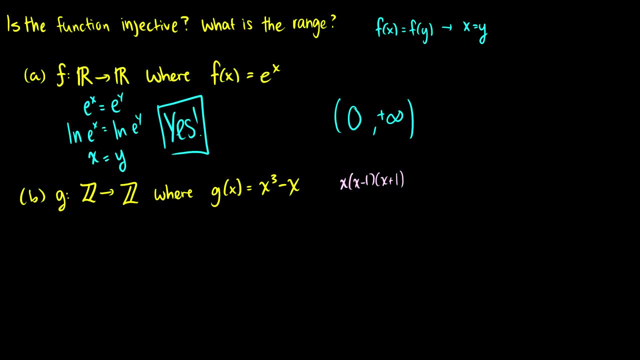 maybe these aren't going to be injective. maybe we can find two values that are equal to each other. in fact, when I see here I'm, when I factor this, it's kind of telling me to look at the values of 0, 1 and negative 1, so we just have to show. 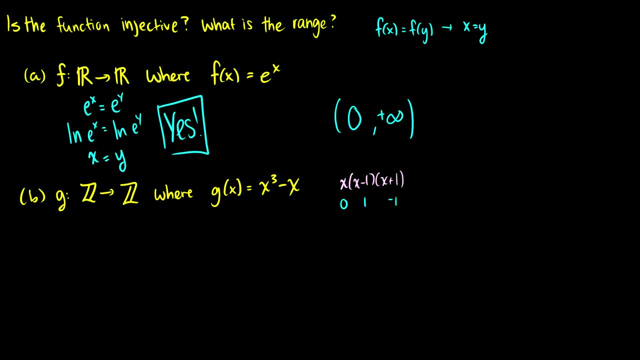 that two of these are equal, and then we'll know it's not injective. so let's take a look here, let's take a look at G of 0 and let's take a look at G of 1. so G of 0 is going to be 0, cubed minus 0, and 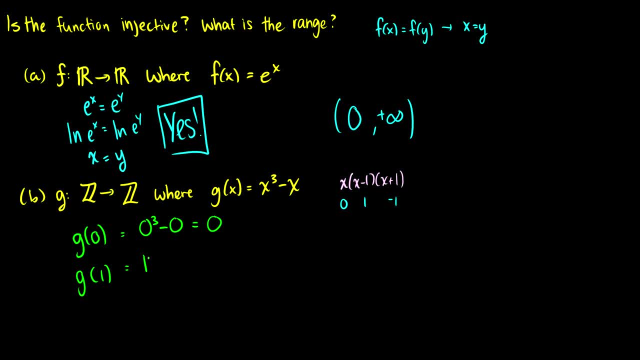 that's equal to 0, and G of 1 is going to be 1 cubed minus 1, which is equal to 0. so we know that G of 0 and G of 1 are equal to each other. therefore, we have 2. 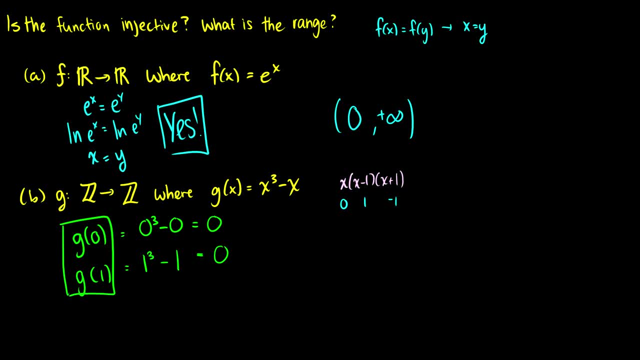 elements in the domain mapping to the same element in the codomain. therefore, it is not injective. okay, and you can also check here: G of 1, G of 0 is equal to 0 and the negative value is not injective. so it's g of negative one, which would end up being negative one, minus negative one, which also 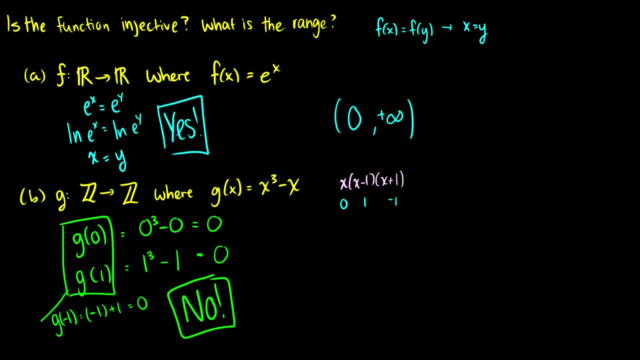 equals zero. So we can see that there's actually three elements in the domain that map to the same element in the codomain. So what's the range of this? Well, we're in integers, so we can't use an interval. Therefore, our best bet is to use set notation. So our range is going to be the set of. 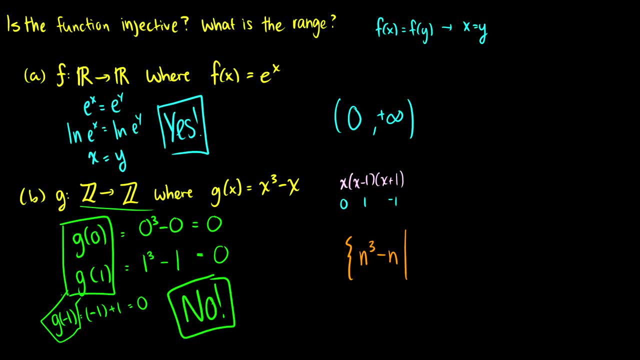 n cubed minus n, such that n is an integer And this will produce all of the outputs. I know it's kind of cheating because you see, wait, that's the function right there, But this is the range. This is the best description of the range you can give. Okay, so that's the first question. 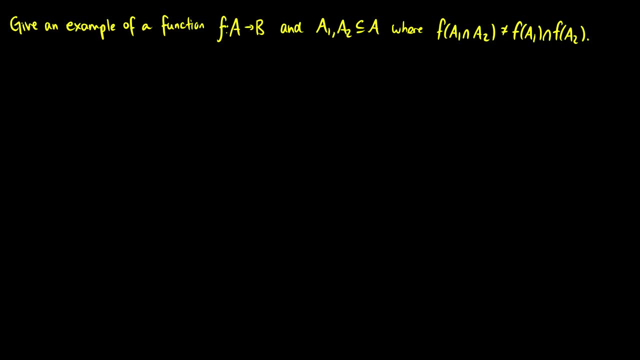 The second question. I want to give an example of a function f from a to b and I want to give two subsets of a to b. So I'm going to give a function f from a to b and I want to give two subsets. 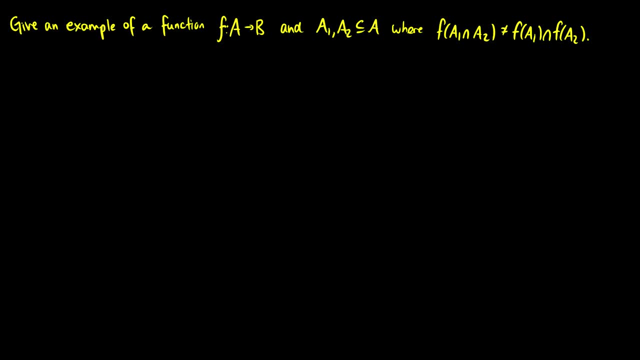 of a to b. So I'm going to give a function f from a to b and I want to give two subsets of a to b, a1 and a2, where f of a1 intersection a2 is not equal to f of a1 intersection f of a2.. 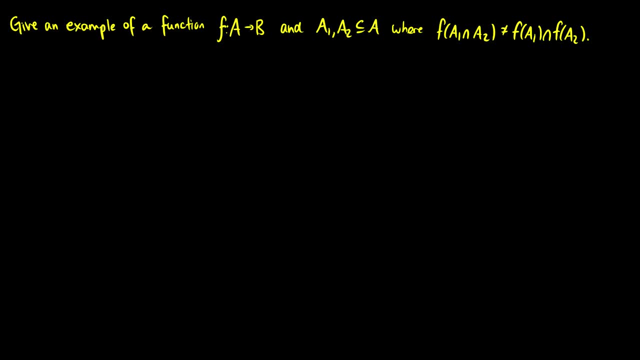 So what I mean here is, if I take the intersection of the two subsets, it gives a different set of values than if I take the function in each of the subsets individually and then take the corresponding values and take the intersection. So a nice way we can do this. 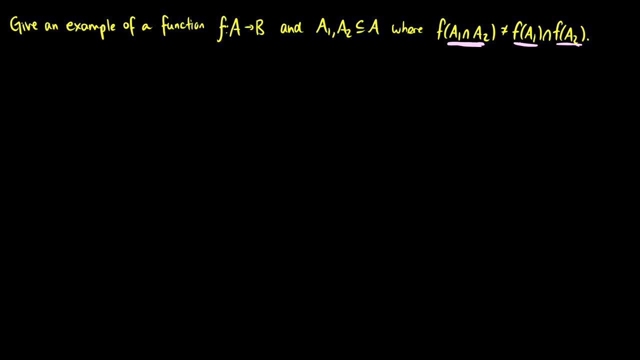 is. we can say, okay, let's let a equal two elements and we're just going to put one element in each subset. So let's say a equals 1 and 2.. We're going to say that a1 is equal to the set. 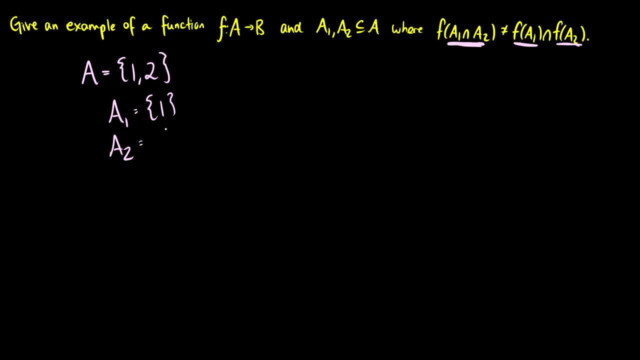 containing 1, and a2 is equal to the set containing 2.. So the nice thing about this is that f of the intersection of a1 and a2 is equal to the set containing 2.. So the nice thing about this is that. 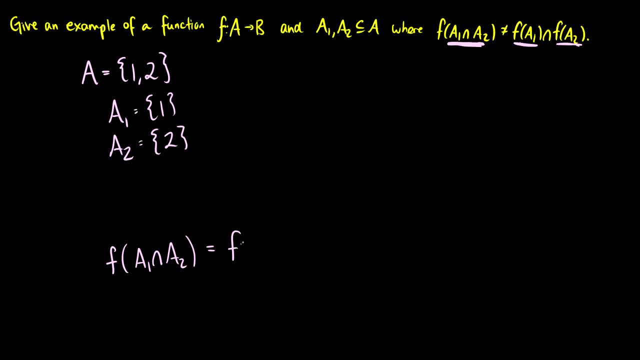 f of a1 is going to be the empty set. So this is f of the empty set. And when we put the empty set into a function, what do we get out? Well, we get the empty set back. So now we also need to figure. 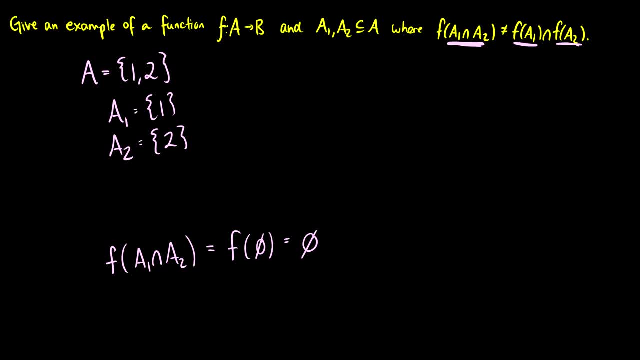 out what f of a1 and f of a2 are. So we need our codomain b, and what would be nice is if we could get 1 and 2 to map to the same thing. So we're going to say that b is just 0. Okay, and we're going to define that f of a1 is. so I might. 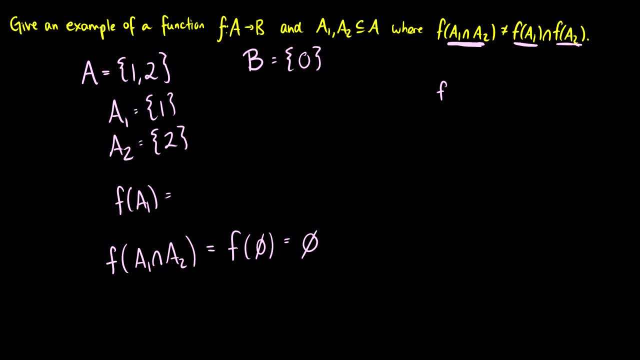 define this a little bit more clearly on the right here. So we're going to say that f of 1 is equal to 3, and f of 2 is equal to 3.. So f of 1 is equal to 3, f of 2 is equal to 3.. So when I put f of 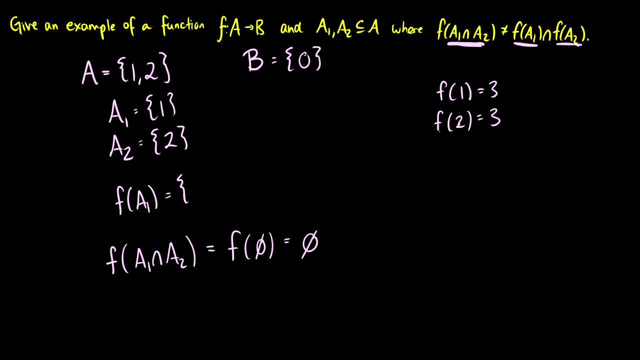 a1 in, we're going to get the set containing 3 back, And then when I put f of a2 in, we're also going to get the set of 3 back. So this means that f of a1 intersection f of a2 is going to.